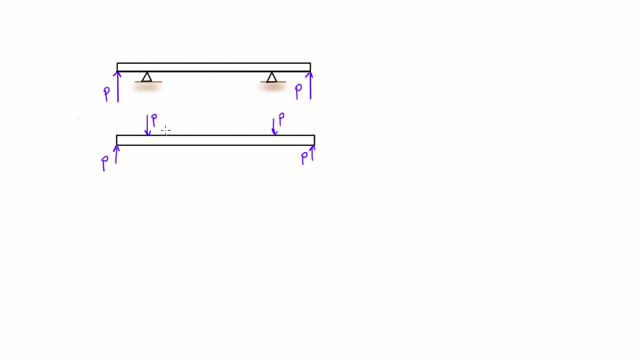 section here from the end of the beam with the first reaction. but once we pass this reaction here, we're not going to be having any more shear here, because if we were to draw our free body diagram, we would have p pressing up somewhere over here, we'd have p pressing down and then 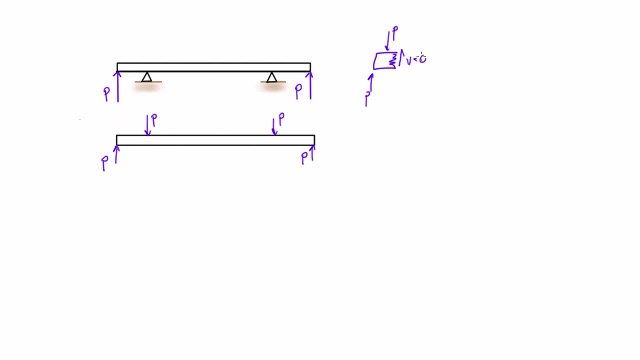 for our shear force v, it would just shear would be equal to zero. So that's true for this whole section in here. So as far as the beam is concerned, all the middle section of the beam sees is just applied moments. and they would be going like this because these force couples basically just 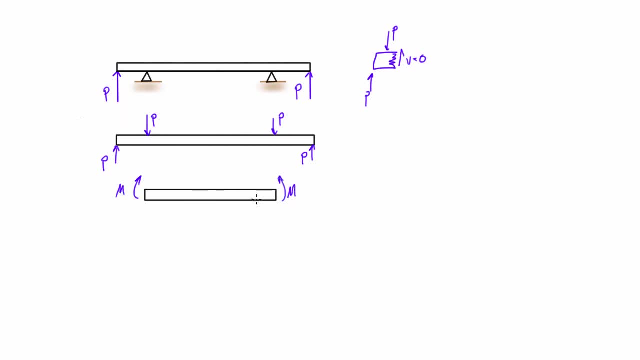 exert an applied moment on the middle section, just like that and for all. the middle section knows that's what's going on. Now, if we have applied moments like this, if we were to draw a little free body diagram with a virtual cut in it coming from the left-hand side, 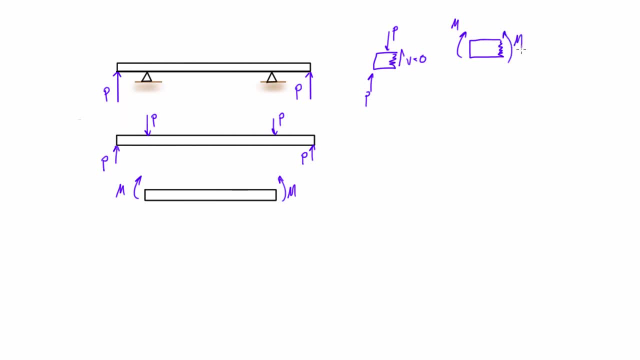 we would have our applied moment and then we would need an internal moment going like that to cancel that out. And if you remember, from statics, this is the positive sense for an internal moment. so that would be positive. or if we drew it from the other. 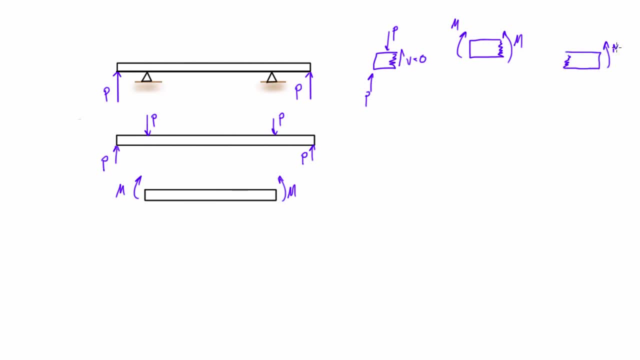 side where we took that cut, where we have a moment like that, when we have a moment on the left-hand side going clockwise, that was also the positive sense for our moments. And so when we have moments like this, that when we apply them, you imagine if you grab a ruler or something and you apply moments, 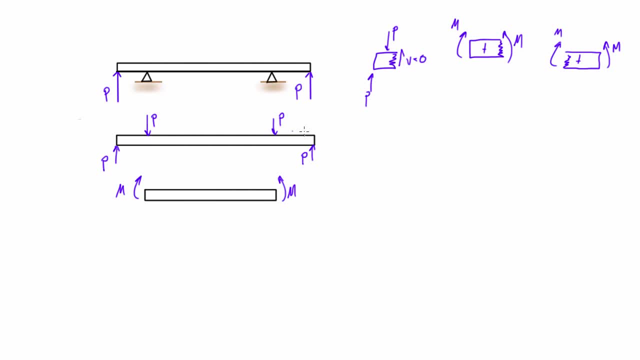 like that. it's going to sag down in the middle or the concave side will be on the top. We call that a positive moment because it's giving us that positive internal moment. If we had the applied moments going down like this in the opposite direction, we would be getting a negative internal. 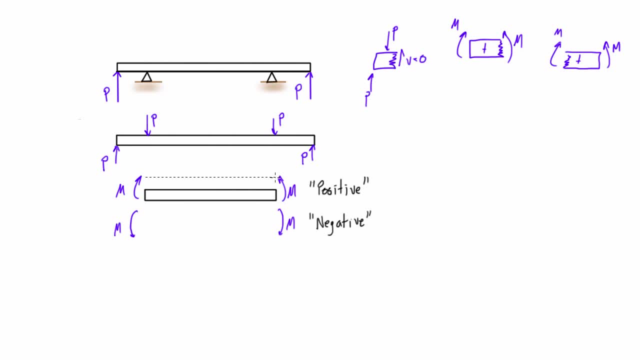 moment. So if we define the section here, the section that is in pure bending, to have a length of L, then we know it's kind of obvious like that, when we talked about using bending a ruler, you know that it's going to want to have the tendency to bend down like this. So really, after we apply, 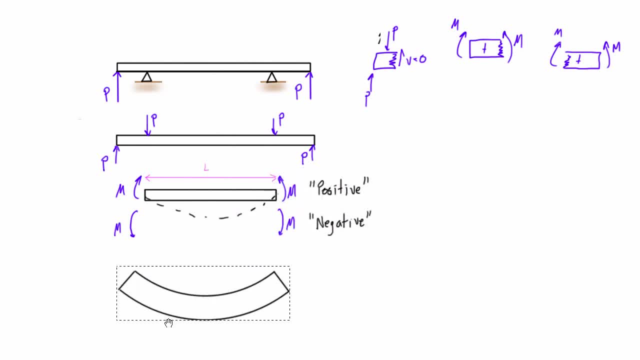 these moments we're getting a final shape that looks something like this. But if we bend an object with actual depth like this, you can see actually that this line here is shorter than this line And basically what we've done is we've taken an original length of L. 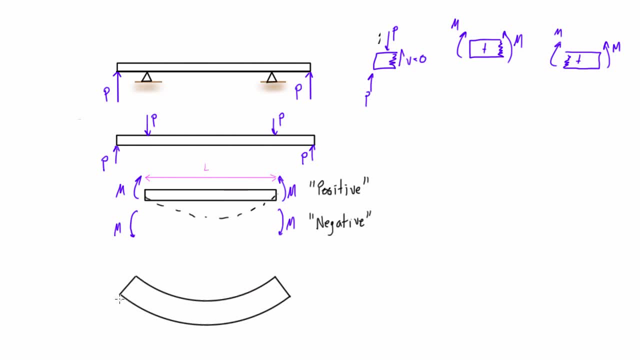 and the top has compressed a little bit and the bottom has stretched out a little bit to get this final shape. Now, if the top is shorter and the bottom is is longer, that means that somewhere in the middle there has to be the exact length of L, and it turns out that for a, it turns out for: 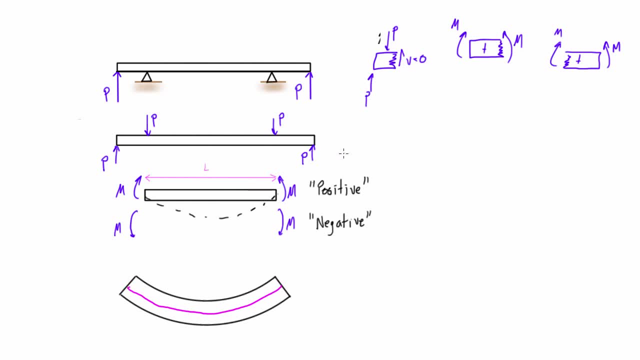 that a for a rectangle. if this is a beam of the rectangular cross-section that it has, that line is right in the middle. So for a rectangle, like I said, it's exactly in the middle, halfway from the top, halfway from the bottom. But if we have different shapes that aren't symmetrical, we can. 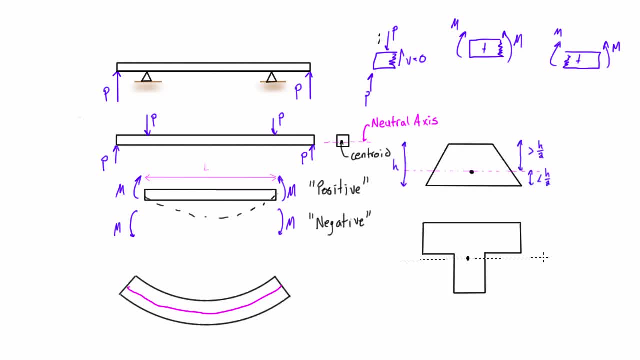 get the neutral axis. So that's what we're going to do. So we're going to go ahead and we're going to get the neutral axis appearing either close, you know, closer to one end or closer to the other end. But it doesn't matter exactly what the cross-section is, whether it's a square or a trapezoid or a. 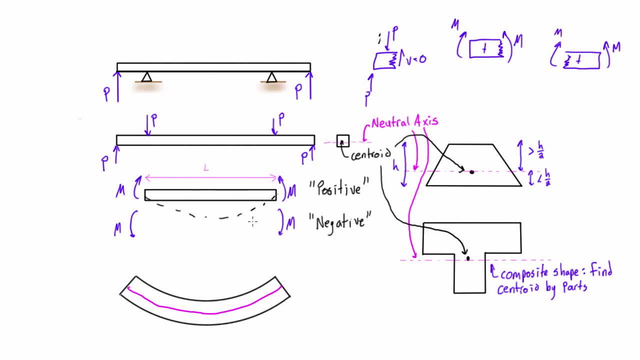 T-shape or an I-shape. If we're applying a moment like this so that we get a positive internal moment, then where, no matter where the neutral axis falls, if it's exactly halfway or if it's closer to one end or closer to the other above the neutral axis we're going to be getting. 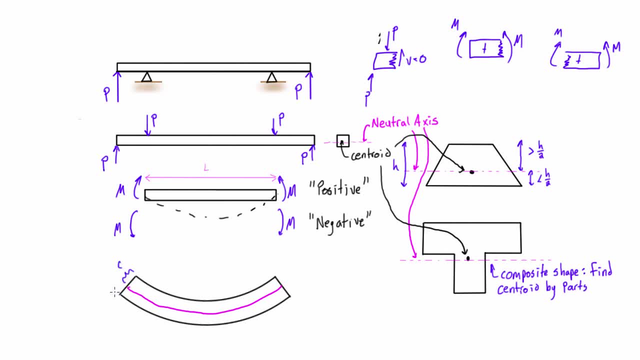 compression and below the neutral axis we're going to be getting tension, And this is because the top half of the member, or the top part of the member here is really is compressing. it's getting shorter, so we're finishing here with with lengths less. 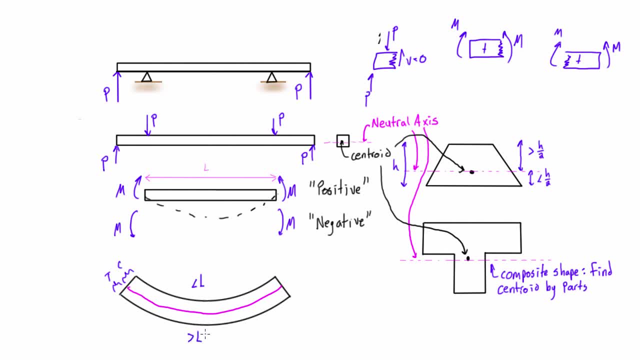 than L, and down here it's elongating, so we're getting lengths that are greater than L. Now, if we had the a negative internal moment, then this would be flipped. We would have tension on the top and compression on the bottom. But compression and tension are really measurements of a force, or 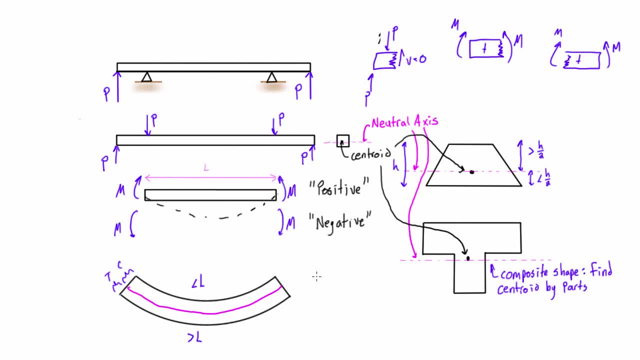 a force when we're talking about length and we're talking about changes on length. So if you think about what the expression for strain is, we have the displacement over the original length. Now, if you recall, we're talking, we call this positive if it was in tension and negative if it was in. 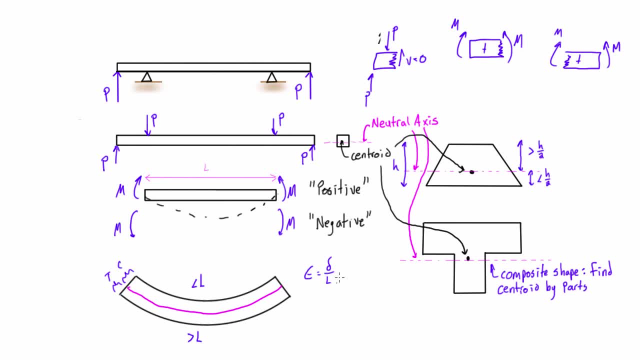 compression. but really what we want to do is we want to relate this into the force or the stress so we can actually confirm that, yeah, we're getting compression and tension. So we have Hooke's law, which was the normal: axial stress is equal to the actual force. So we can actually confirm that, yeah, 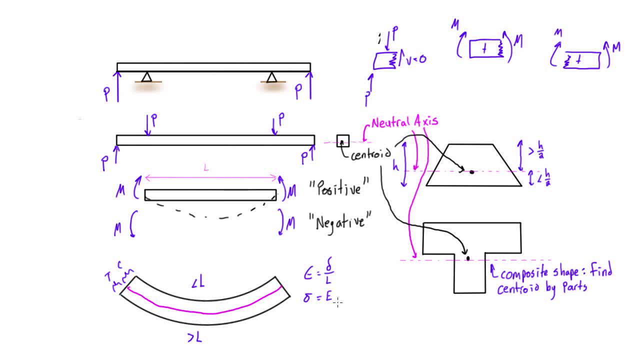 we're getting compression and tension. So we have Hooke's law, which was the normal axial stress is to the modulus of elasticity times the strain. So if we just rearrange that for strain we get that's equal to stress over e and stress, if you remember, is just a measurement of force over area. 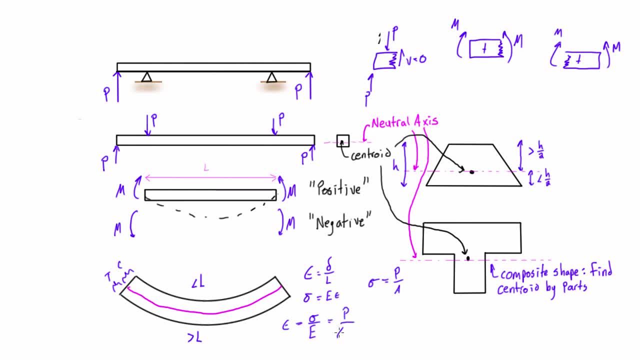 so we're getting p over a, e basically. So by applying these moments on the end, we're actually creating strain by changing the deformations here, by either shortening the member or lengthening the member, and when we do that we induce an internal stress. So basically, all you need to 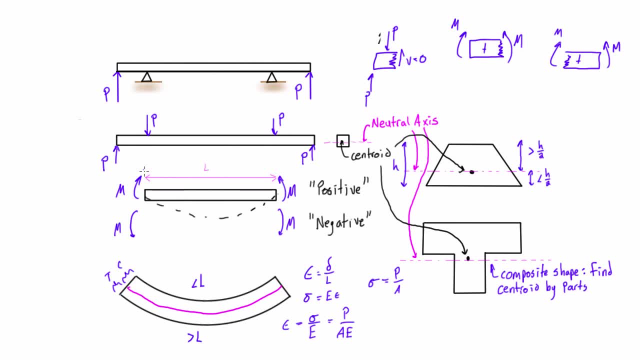 take from this is that when we have a positive internal moment caused by applied moments like this, that the normal stress and strain are going to be compressive above the neutral axis and tensile below the neutral axis. 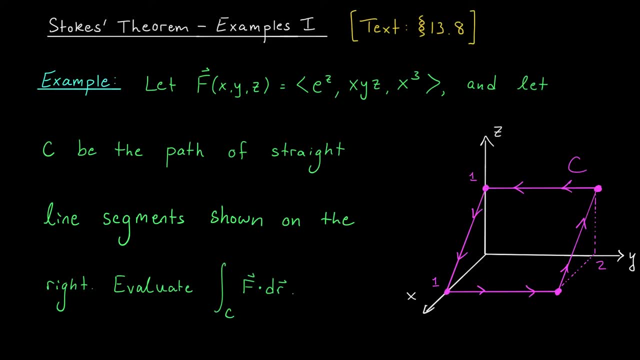 Welcome back folks. Today we're going to be looking at the following example. We're given a vector field f of x, y, z- equals e to the z, x, y, z, x cubed- and a path C consisting of straight line segments shown on the right. So our path seems to be forming this: 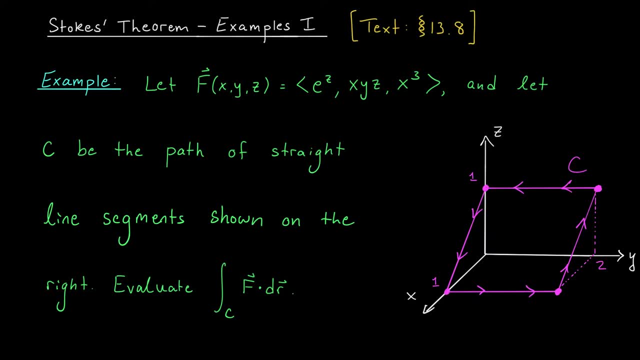 rectangle in R3.. We'd like to evaluate the line integral of our vector field f along the path C. Hmm, Now, at a glance this problem actually looks pretty involved. After all, our curve C is made up of four straight line segments, So does this mean we have to compute four separate line? 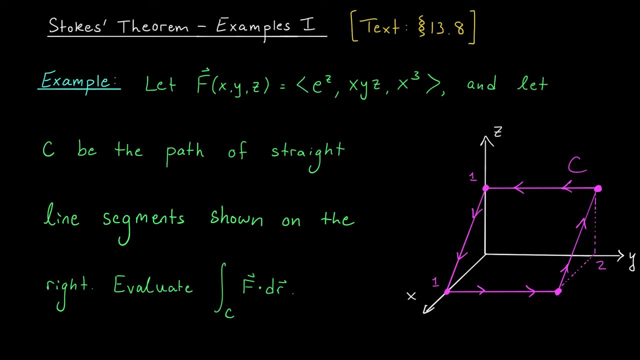 integrals and then add the results. Well, maybe We were able to avoid this in the past using Green's theorem, but that result doesn't apply here. Green's theorem only works in R2 when we're dealing with curves in the x- y plane. But wait a second. We have a three-dimensional generalization.